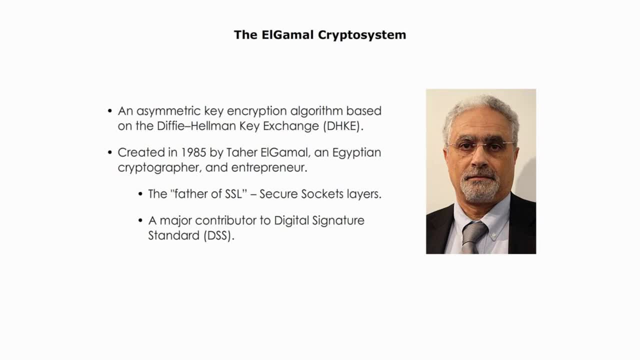 The Agamal algorithm was created in 1985 by Tahir Agamal, an Egyptian cryptographer and entrepreneur. He is considered as the father of SSL. SSL stands for Secure Socket Layer. SSL encrypts data between the user and web server, and thus protecting the user's privacy. 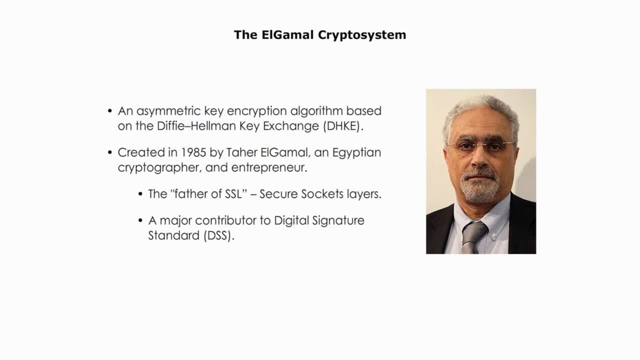 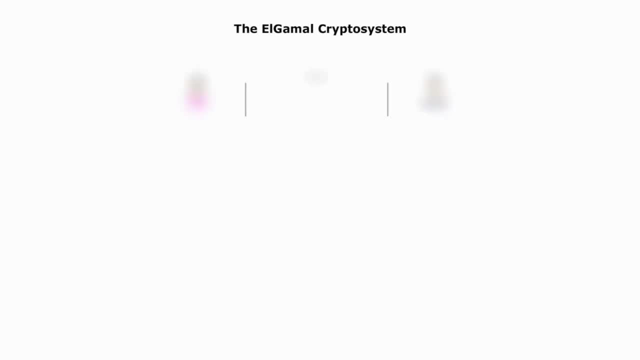 He is also the major contributor to Digital Signature Standard. Here is the scenario: Bob wants to send a message to Alice, Bob is the message sender and Alice is the message receiver. They agree to use Agamal for encryption and decryption. Keep in mind: the public key system always starts with the message receiver, who is responsible for public key generation. 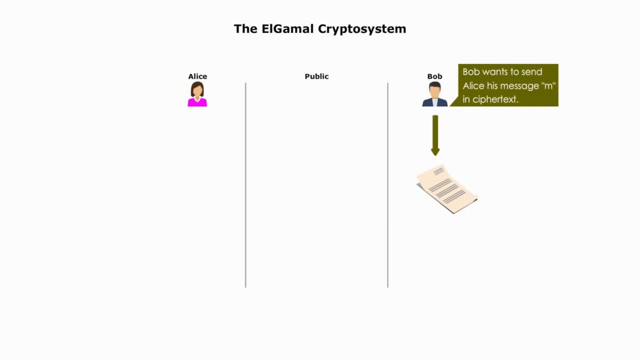 The process of Agamal algorithm consists of three major steps. Step 1. Key generation by Alice. the message receiver, Alice will generate a pair of keys: public key and private key. She sends the public key to Bob. She keeps the private key. 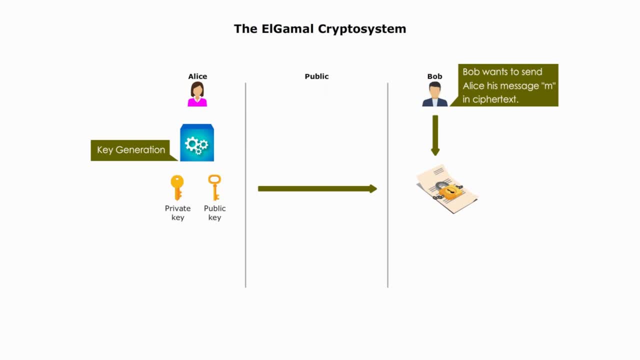 These two keys are mathematically related. Step 2. Bob, the message sender, will use Alice's public key to encrypt his message and send the encrypted message ciphertext to Alice. Step 3. Alice uses her private key to decrypt Bob's ciphertext. 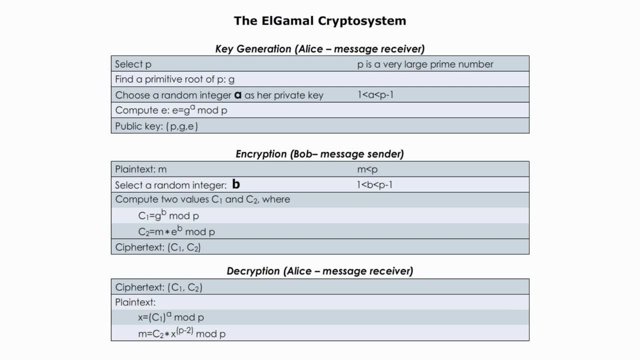 Alice uses her private key to decrypt Bob's ciphertext. Here I will use math formulas, and it could be, or it must be, very boring and tedious, which is the nature of a cryptosystem. But once we go through these formulas and once I demonstrate the whole process again by plugging some real simple numbers, everything would make perfect sense. 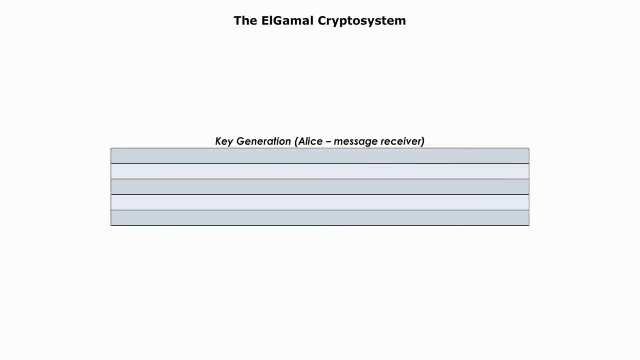 Now let's see the details step by step. Step 1. Key generation by Alice. The following is sub-steps. And first select p. p is a very large prime number. Then find a primitive root of p g. In my last video I talked about how to get a primitive root of p. 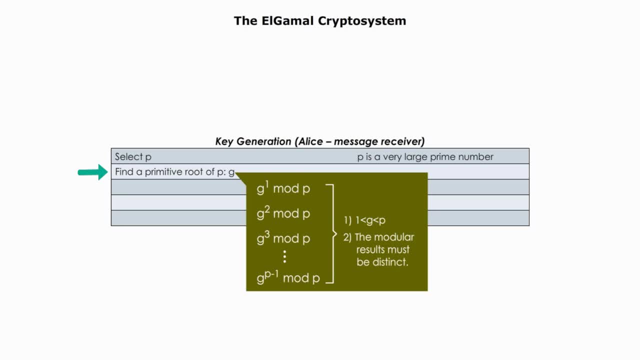 So if you don't know how to find a primitive root of p or how does it works, please refer to my last video about how to find a primitive root. Then choose a random integer, a as h. This is her private key, Where the private key a is bigger than 1 but smaller than p-1.. 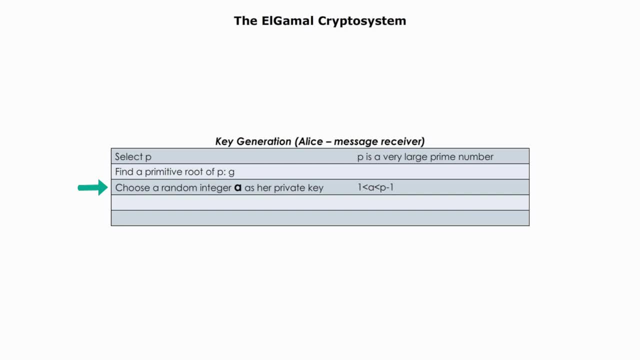 So again, a is a random integer, not necessarily a prime number. The next compute e. So the formula is: e equals g to a mod p. And then Alice gets the public key, which is p, g and e. So three values as a public key. 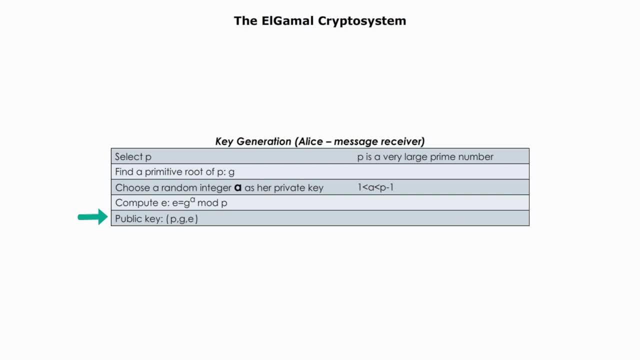 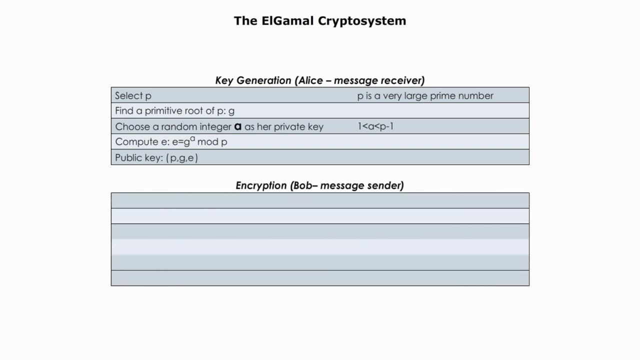 And she will send the public key to Bob. Step 2. Encryption by Bob. So suppose Bob wants to send the plaintext m. So m must be smaller than p in terms of value And select random integer b. So that's a random integer b. 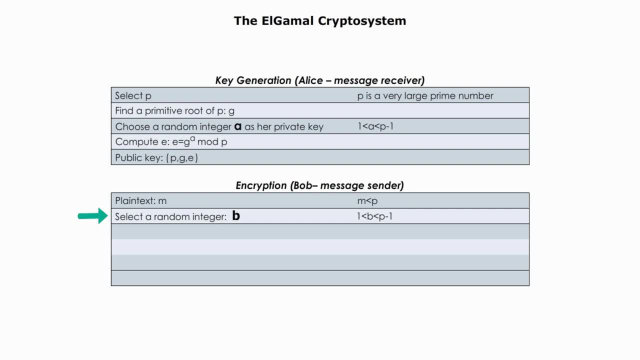 And b is bigger than 1 but smaller than p-1.. Next compute two values, c-1 and c-2.. Where c-1 equals g to b mod p, c-2 equals m times e to b mod p. And then he gets the ciphertext c-1 and c-2. for the plaintext m.